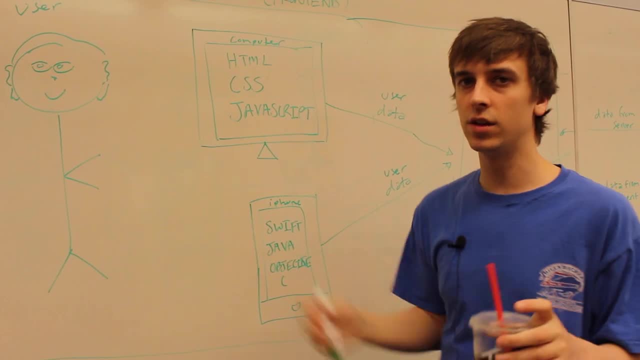 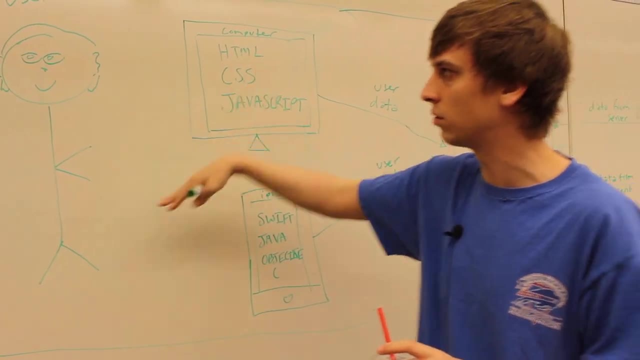 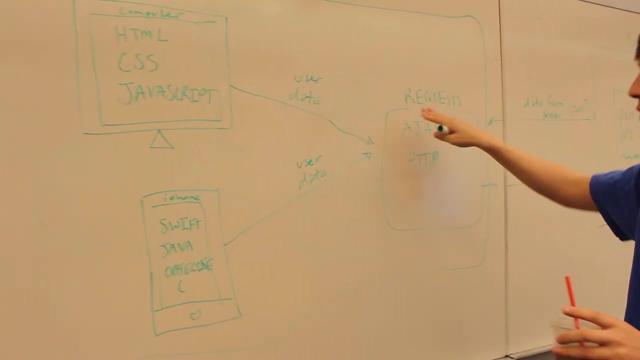 from the user. what happens to the input? so the input, maybe the users like: I'm creating you know it says create an account on Facebook. so the users like: okay, they type in their email and their password, right, what happens to the email and password? well, the email and password from these devices. it gets sent through. 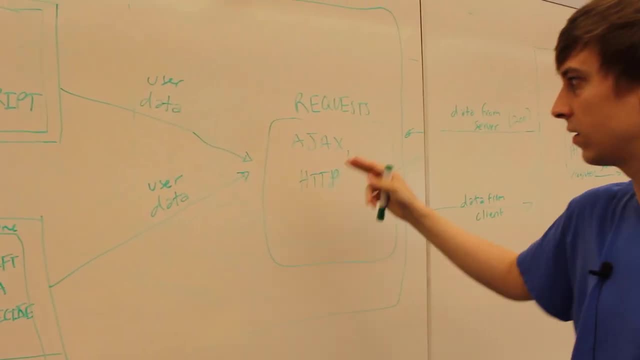 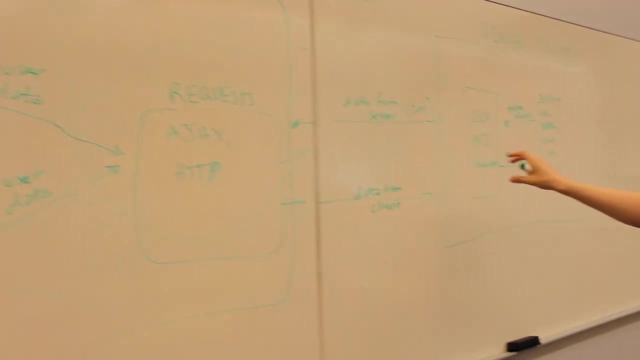 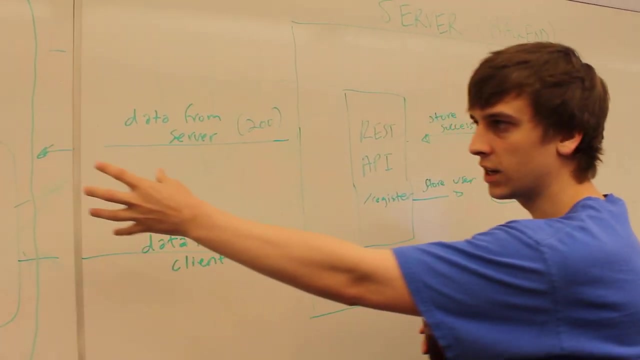 requests, right. so there's these defined requests, like maybe Ajax or HTTP requests, and the data gets sent now to a server side- server side programming, which is a web server or some kind of server that will handle this data. so now we have the user email and password and it is sent through requests to the 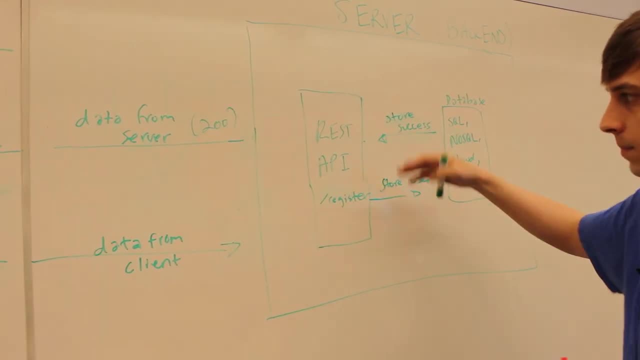 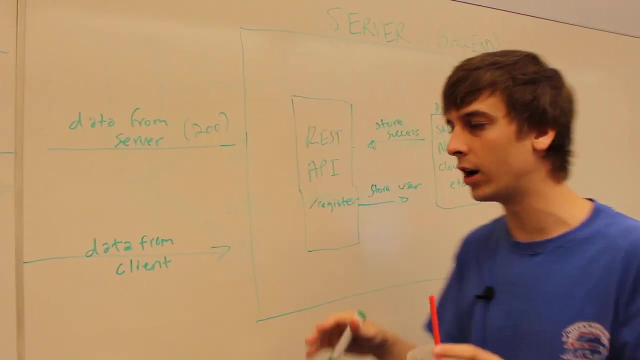 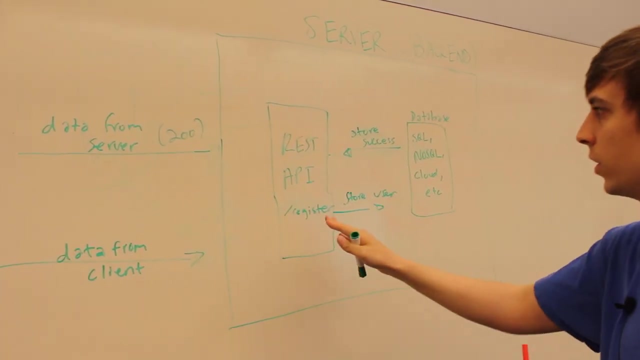 server. now usually what you have is an API or something like that, and these are defined routes that you can send requests to that do things based on the URL. so you know, maybe you have slash register defined in your API and you're like: okay, I have the username, I have the password, so you take the username and 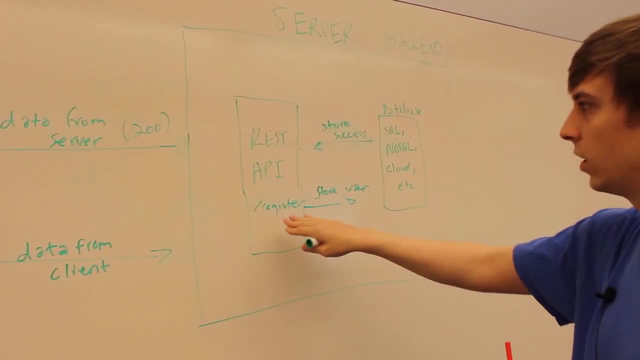 the password and you're like: okay, you have the username, I have the password. so you take the username and the password and you're like: okay, it's hooked up to a database as well. you know, maybe the database is sequel, no sequel or whatever. and we're like: okay, we're gonna store this user in our 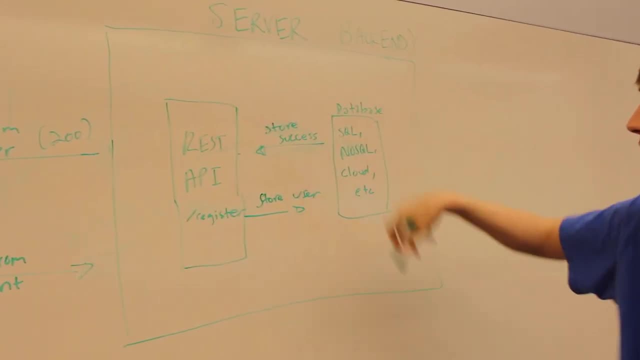 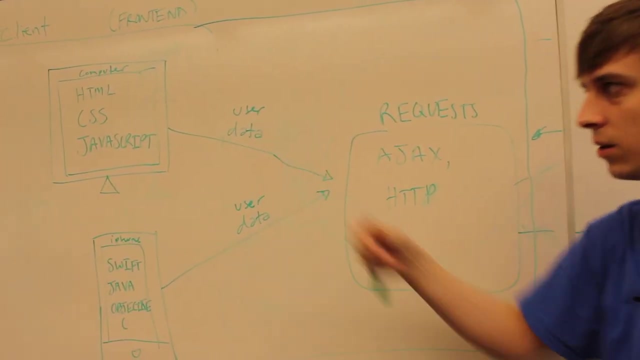 database so the users get stored in the database successfully. the database is like: okay, there you go, success. then you send a 200 back here and then it gets sent all the way back here and then you say you maybe say message to the user like hey, your account was successfully created, and then you log them in, or 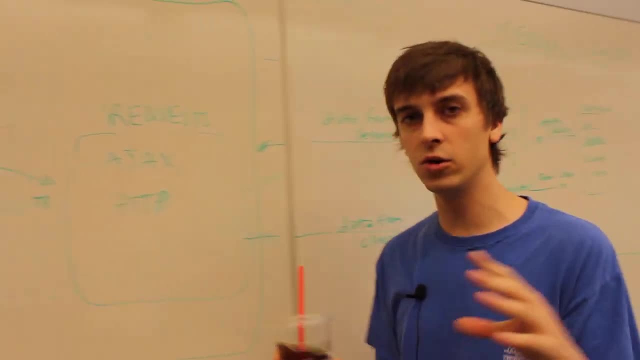 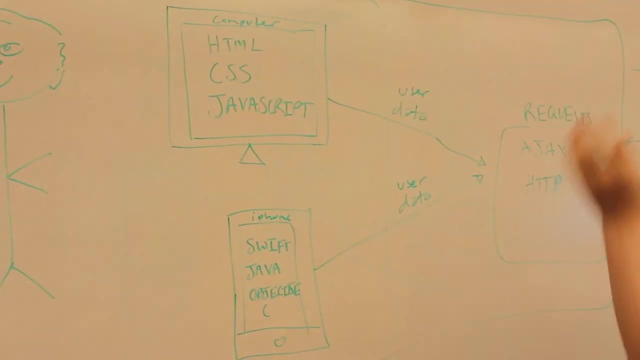 something like that. this is how it works across the board, not just for user login- that's just an example- but for all data, like anything that the user is interacting with, if you need to store it in a database or if you need to do some kind of server-side data manipulation or 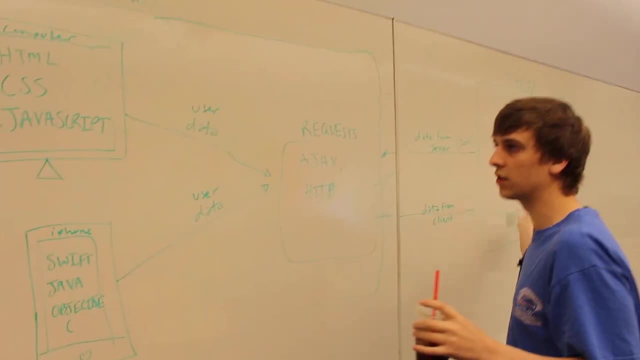 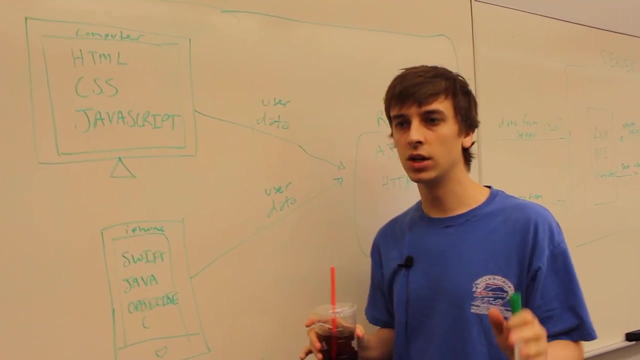 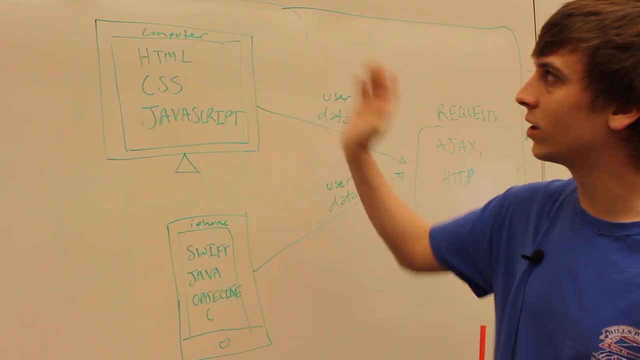 something like that. you're gonna send it over here and then send the results back. this is how you should develop software, for you know simple web app, simple applications. they're not static but they have simple, you know, server-side programming going on. a lot of people just don't understand. you know. 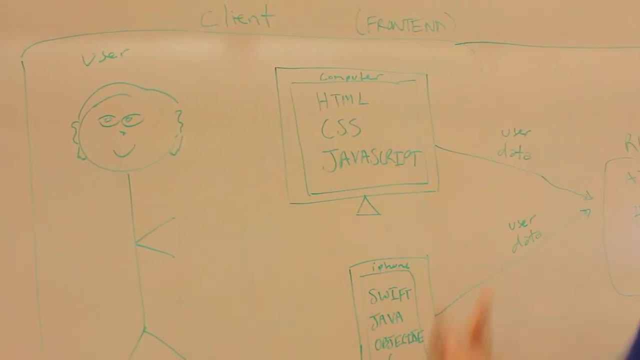 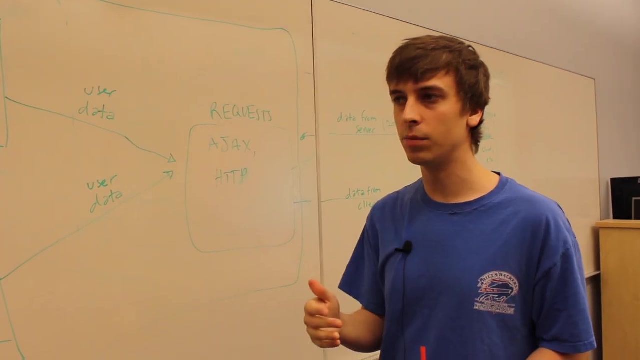 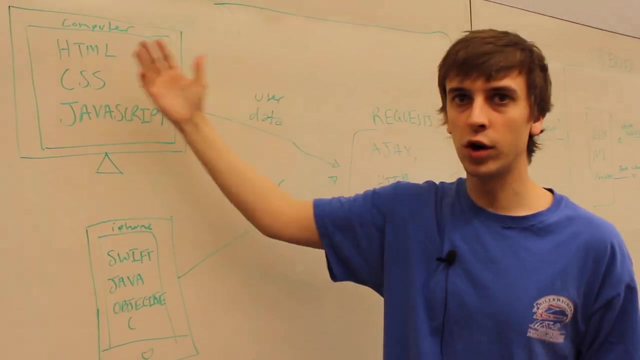 basically the client is the front end. you know front end. the stuff that people see in the back end is the server-side stuff: api, database, big library, manipulation, web sockets and stuff like that. on this side it's very straightforward. you know you could have front-end frameworks. you know react, Ember, Angular, stuff like that, or you. 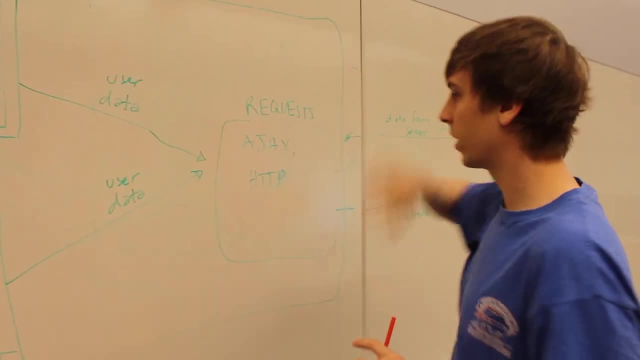 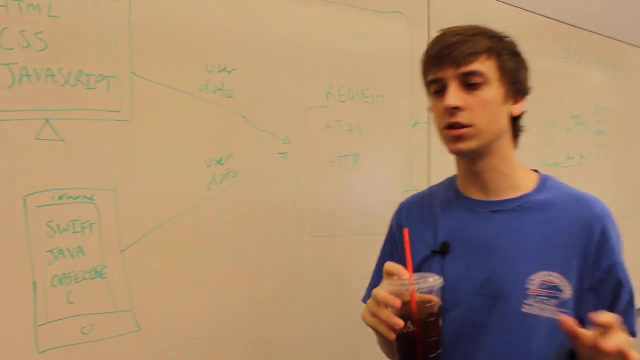 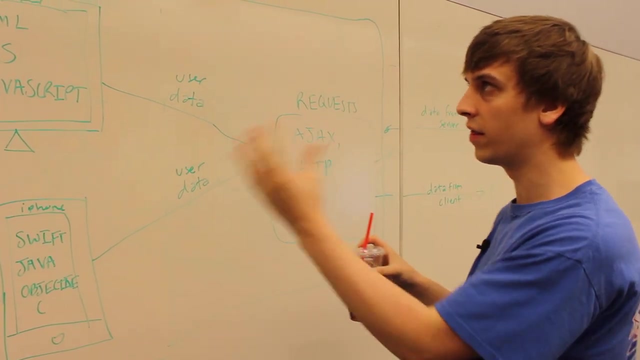 know, mobile frameworks and stuff like that, and you basically just make requests back and forth, simple communication, just back and forth, back and forth. this is the front end, this is the back end. people don't understand that. they need to understand that. Once you understand that, when you go into building a project and know that this 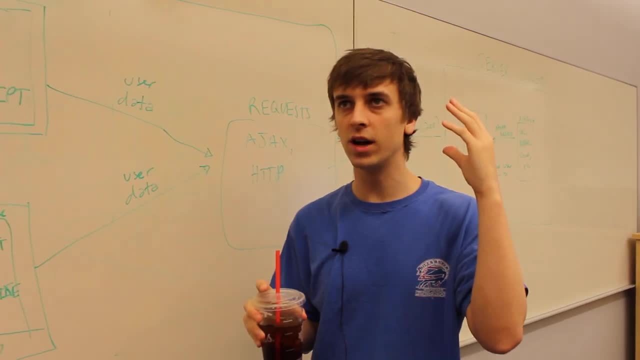 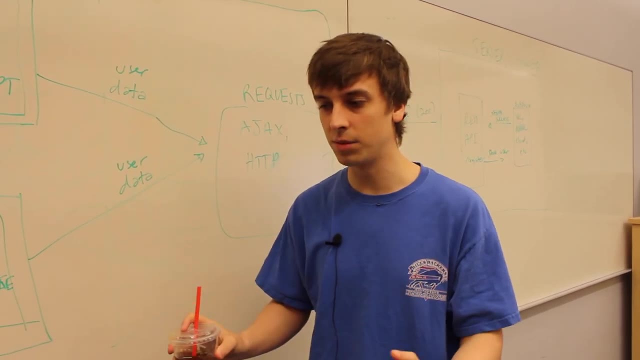 is how you're going to structure things. you're much more organized in your mind. You know what you're doing a lot better. The code comes out better. The end product comes out better, Having it in your mind from the beginning instead of just looking up what's the next step to building. 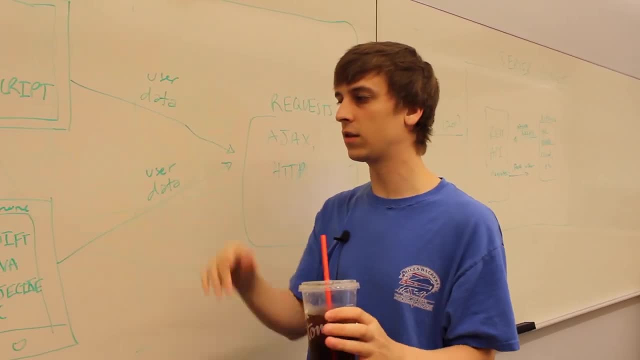 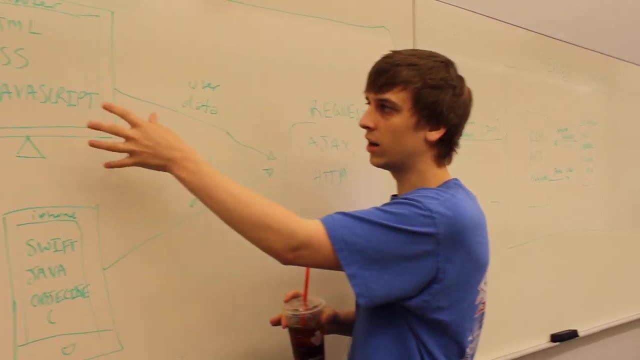 a website. What's the next step after this? Okay, I did this, Now what's the next step? It's going to come out a lot cleaner and you're going to be able to explain it and know what's going on at every stage. If you have an error here, you're going to be like: where's the error? You're not. 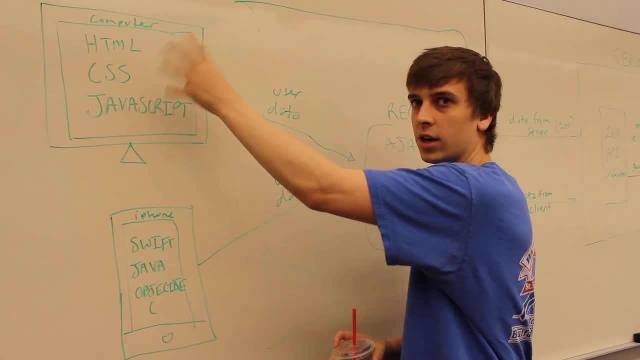 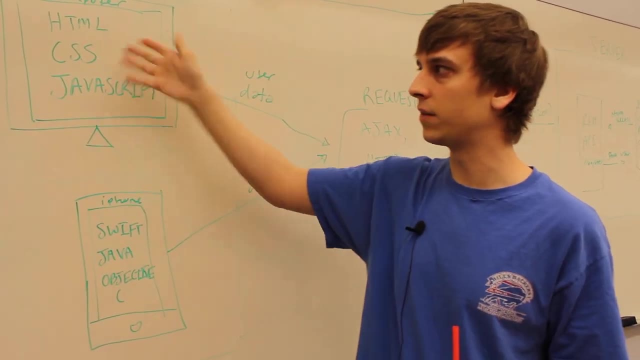 going to be confused about client or server. If it's happening within your front-end code, then you're going to know: okay, the error is in the front-end code. You usually do your debugging in some kind of console, maybe like a browser console or something like that, for front-end. 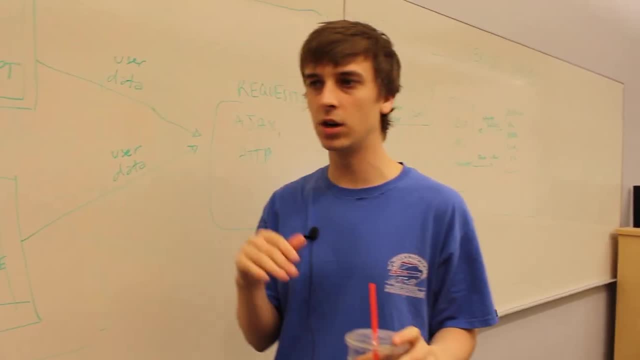 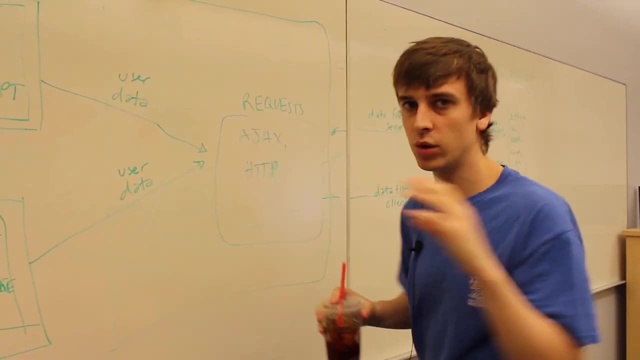 In the back-end you have a server running, maybe on your computer in Python, Java or Nodejs or something. You're going to see that in your terminal or something like that. It's pretty clear once you understand the difference between front-end and back-end and how they communicate. 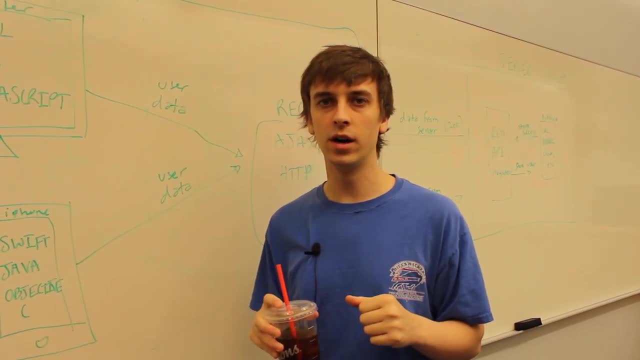 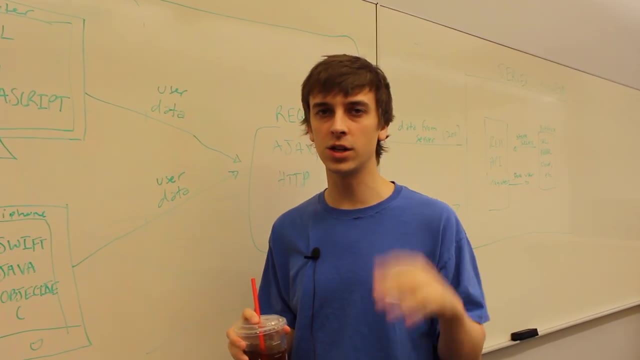 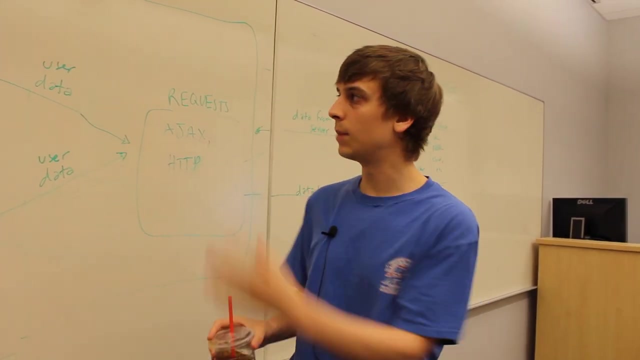 for a simple architecture like this- how to build software and what kind of softwares you can build with this architecture- It just really solidifies your understanding of building software in general. This is one of the most basic things: to understand basic architectures. There's a lot. 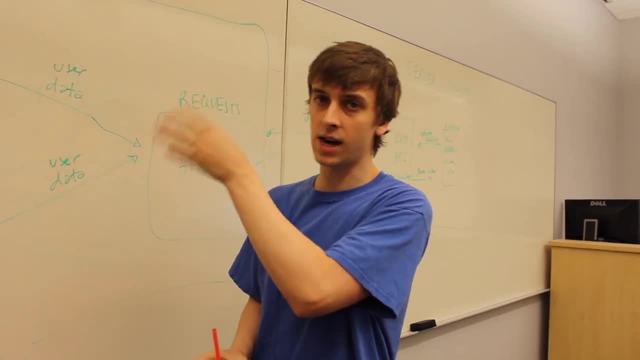 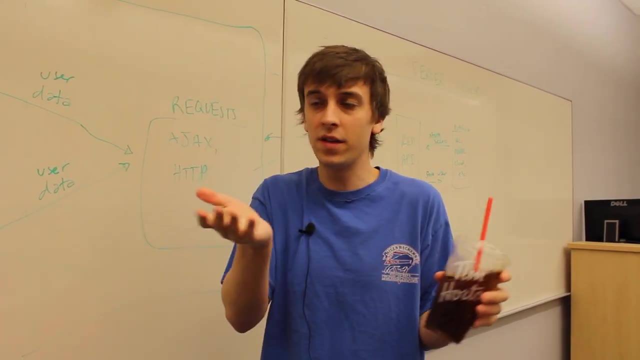 more that goes into that. you can build on top of this, but I think understanding it. a lot of people don't understand this. They don't teach you it. In my web programming class they didn't talk about this at all. I think it's one of the most important things. Hopefully you guys are going to 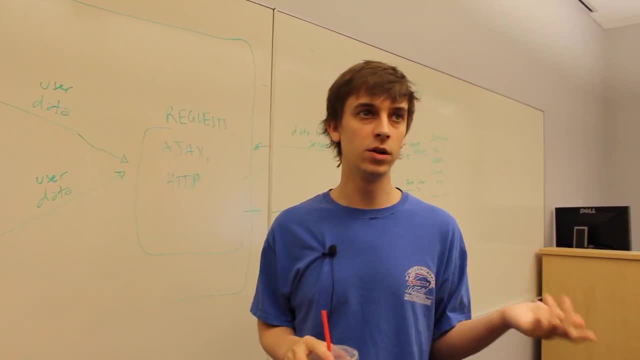 understand it. Let me know, Message me if you don't understand. Comment if you don't understand. Thanks for watching. Yeah, that's it, See you.